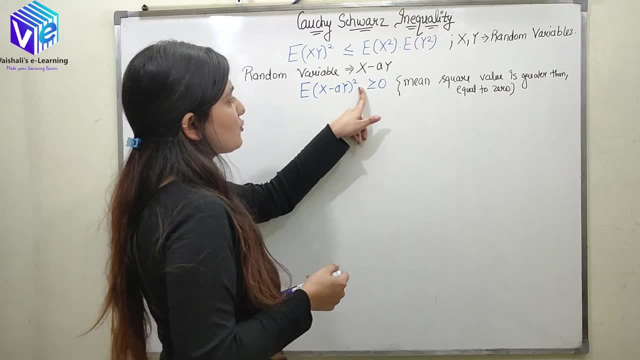 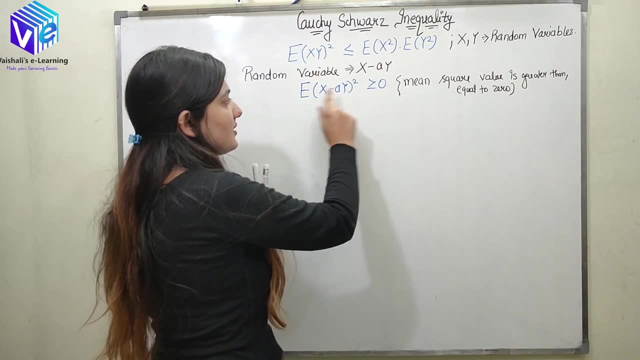 E value is representing the mean and this is the square, So mean square of this random variable. so x minus ay is my random variable now, So its square and mean is greater than equal to 0.. So now, if I expand this, 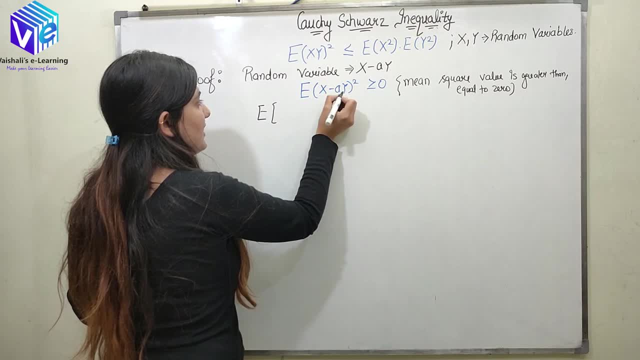 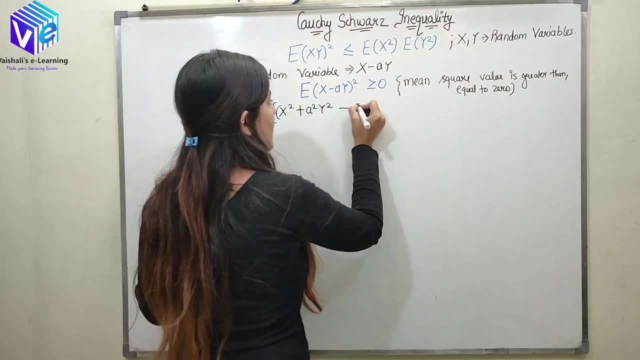 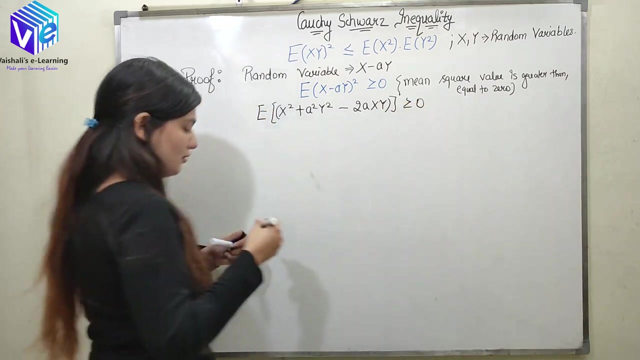 E of xy. So now I can know expectation of random variable x square multiplied by expectation e of. if I expand x minus ay square, I hope you know it is equal to x square plus a square. y square minus 2a, xy is greater than equal to 0 because I know expectation is a linear function. 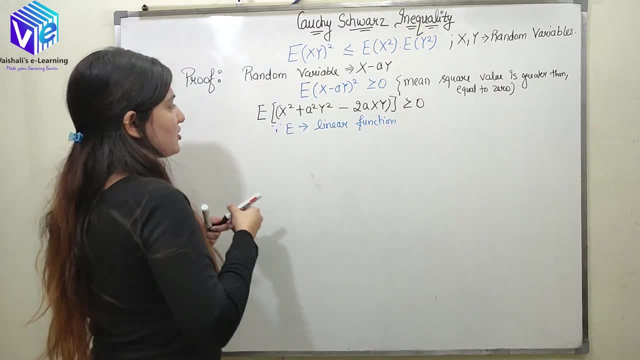 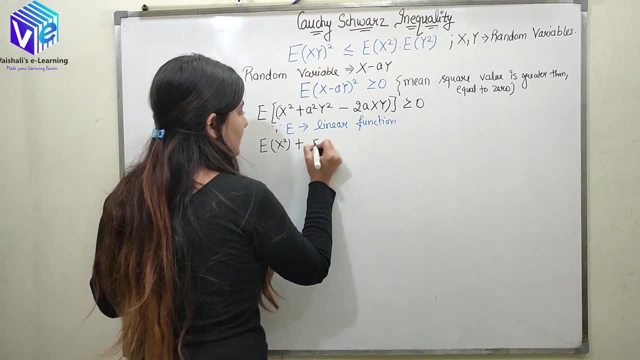 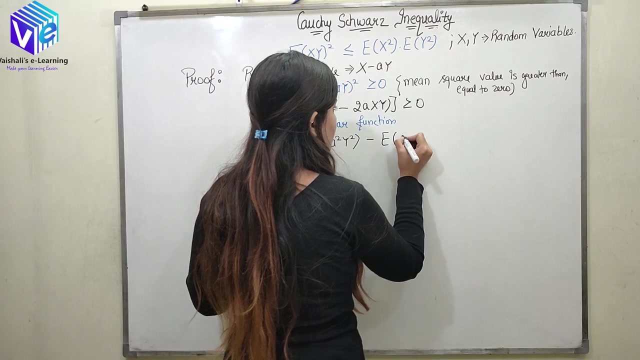 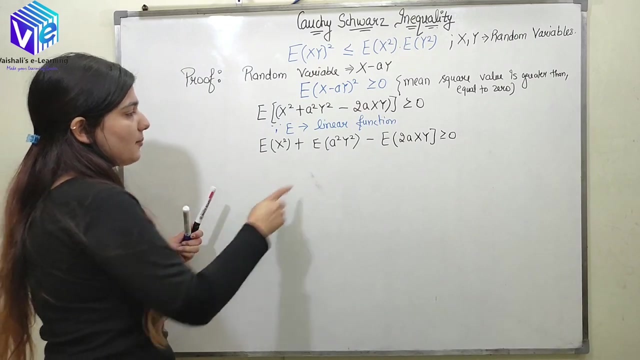 So now in the expansion I can use it. so expectation of x square plus expectation of a square y square minus expectation of 2a, xy is greater than equal to 0.. So now, when I talk about a, a is my constant, so a was this, a is. 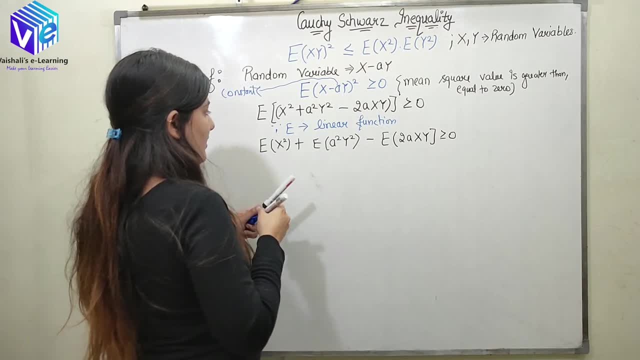 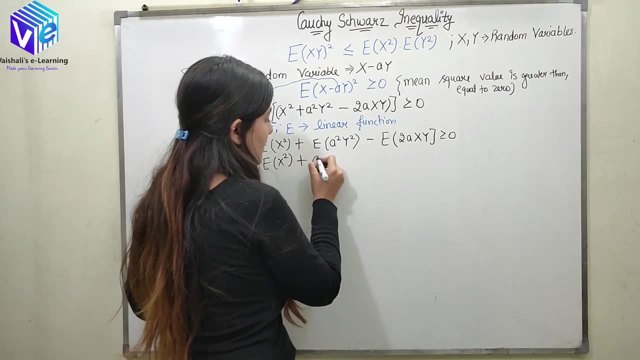 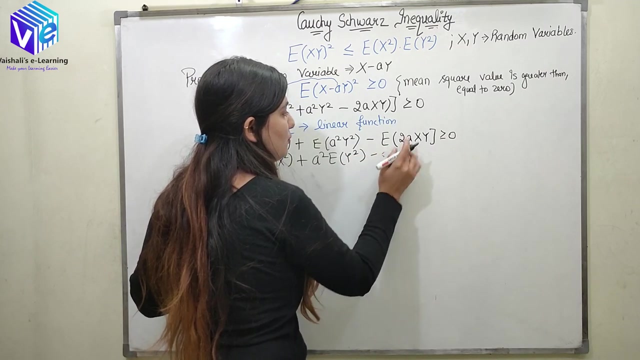 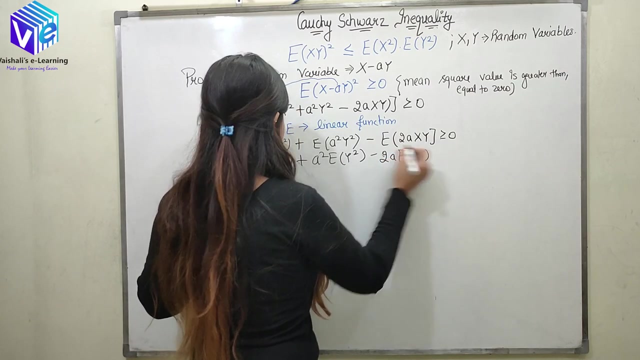 A constant. so now, when I talk about a constant, the expectation of x square plus, this constant would come outside. this is the property of expectation. I hope you remember minus. so now 2a, both are constants, so it will come outside. this is expectation of xy. so now this is greater than equal to 0.. 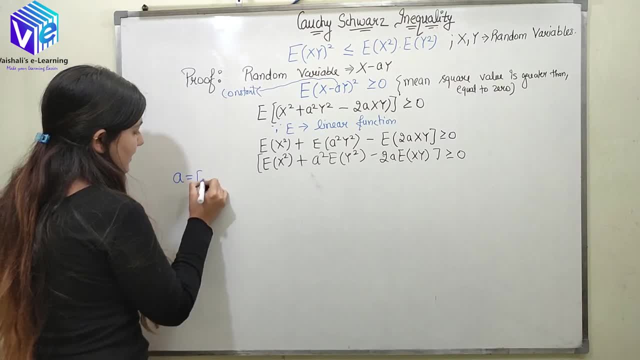 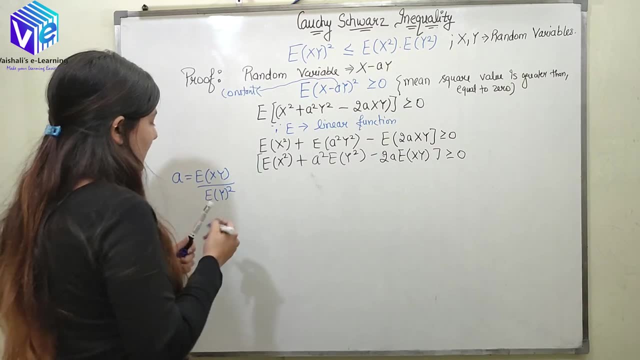 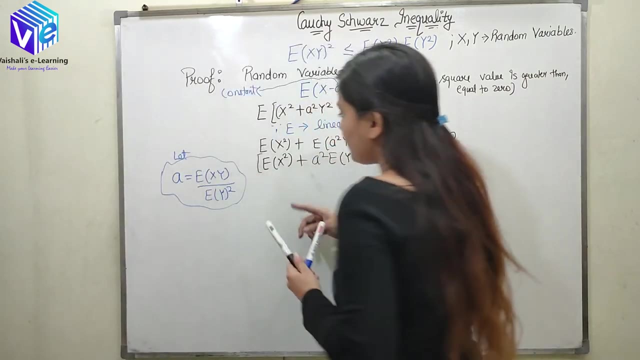 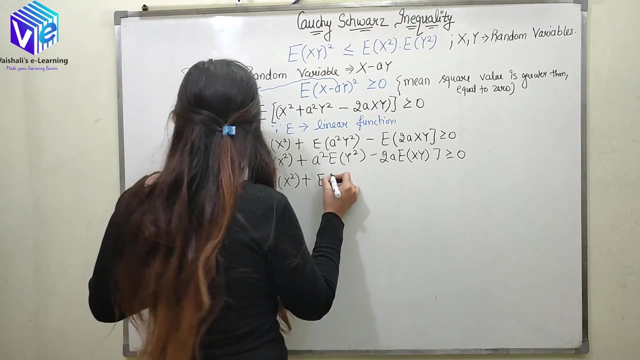 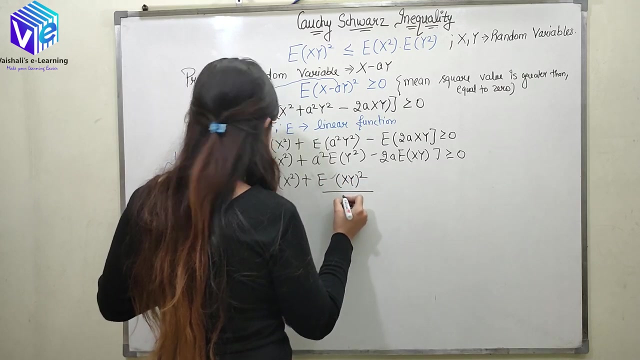 So now I am taking A to be expectation of xy upon expectation of y square. so now when I replace so a is any constant, I am taking the value of a to be this: so when I replace a with this value, it came out to be expectation of x square plus e square, e, xy square upon expectation of xy.